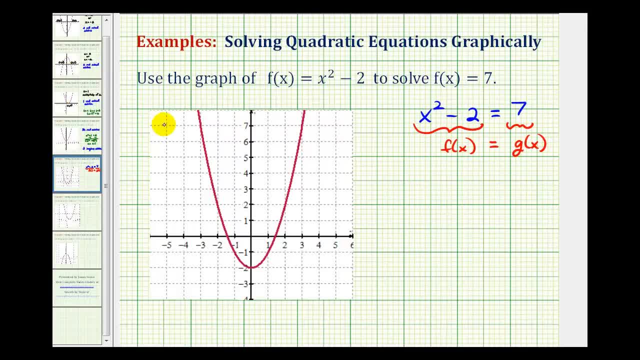 is a horizontal line passing through the y-axis at seven, or this horizontal line. here Again, this is g of x and this is f of x. Graphically we can see they're equal at this point of intersection and at this point of intersection. 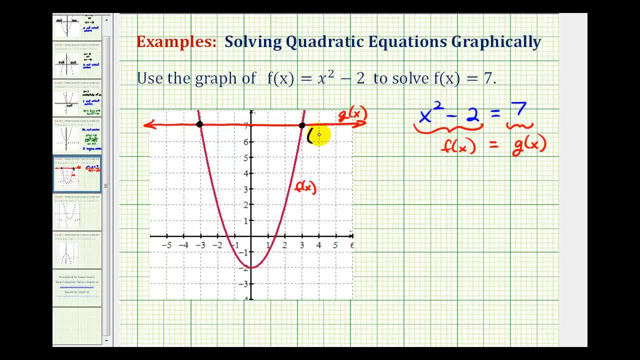 This point of intersection has coordinates three, seven, and this point of intersection has coordinates negative three, seven. So this point is telling us that when x is equal to three, both functions are equal to seven, which satisfies the equation. So one solution is: x equals three. 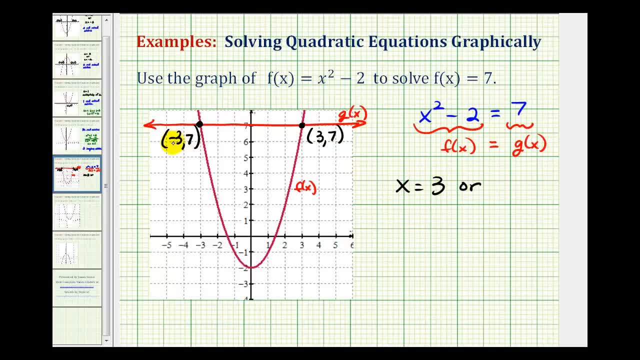 This point here is telling us that when x is equal to negative three, both functions are also equal to seven, which would satisfy this equation as well. So we have two real rational solutions. Let's take a look at another example. Here we want to use the graph of f, of x equals x squared. 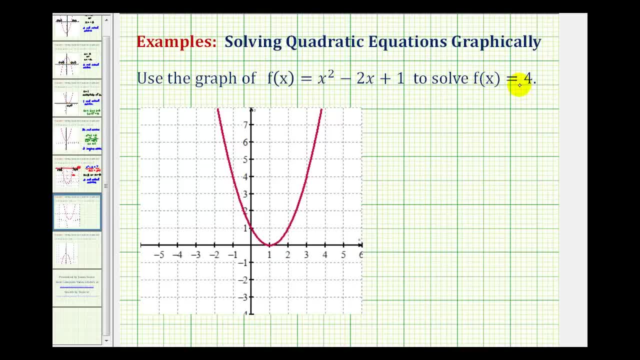 minus two, x plus one, to solve: f of x equals four. So again, we'll start by setting up our equation. We'll substitute x squared minus two, x plus one for f of x. We want to know when this is equal to positive four. 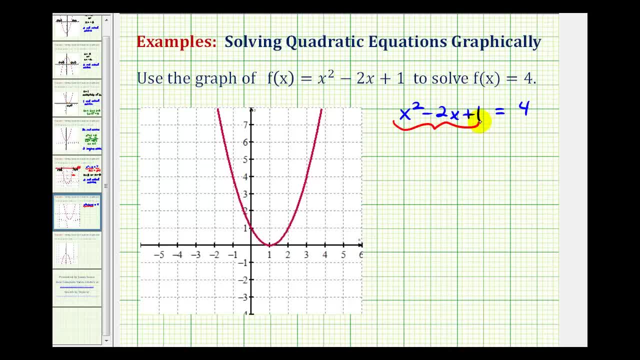 And again, the given graph is: f of x equals x squared minus two, x plus one, which is the left side of the equation. So now we'll graph the right side of the equation as g of x and then determine when these two functions. 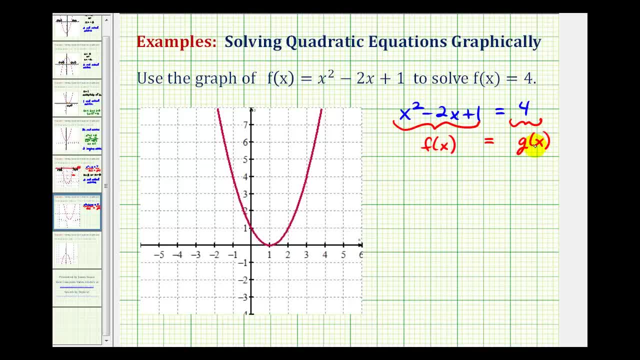 are equal to each other or where they intersect. Well, g of x equals four. again is another horizontal line passing through the y-axis at four, which would be this horizontal line. here Again, this is g of x and this is f of x. 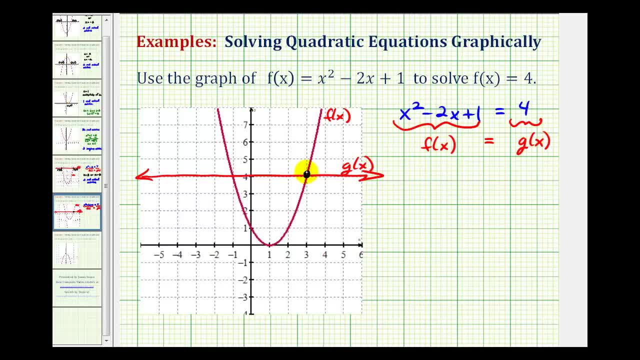 The two functions are equal here, at this point of intersection, as well as this point of intersection, The coordinates at this point of intersection are three, four, and the coordinates at this point of intersection are negative one, four. Notice when x is three and when x is negative one. 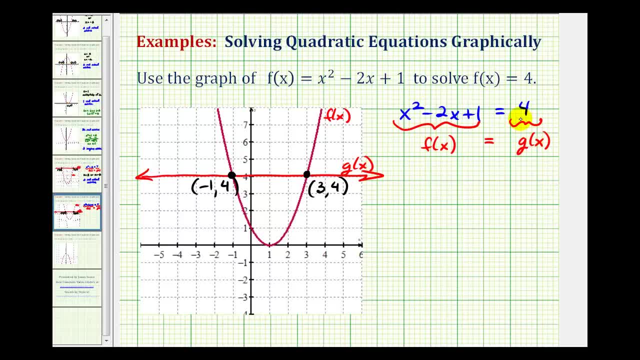 both functions are equal to four, which represent the solutions to our equation. So our solutions are: x equals three or x equals negative one, And again we have two real rational solutions. Okay, let's take a look at one more example. We want to use the graph of f, of x equals. 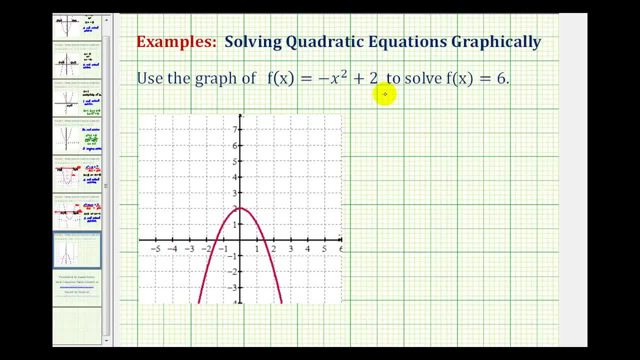 negative x squared plus two, graphed here in red, to solve: f of x equals six. So the equation we're trying to solve would be negative x squared plus two, which is f of x equals six. We're provided the graph of f of x here in red. 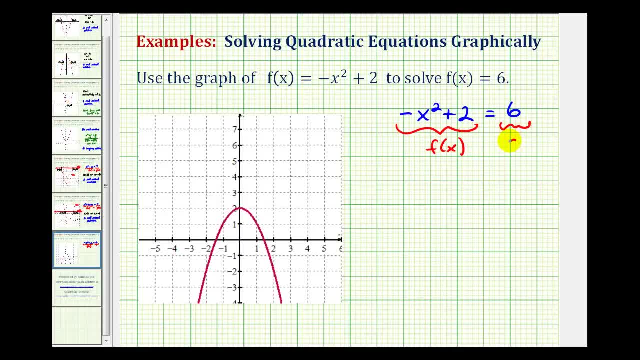 so we'll let the right side of the equation equal g of x and then look for the points of intersection. Again, g of x equals six would be a horizontal line passing through six on the y-axis, or this line here. So here's g of x. 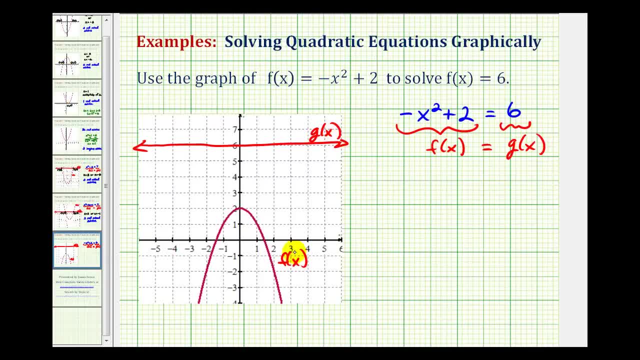 and here's f of x. Notice that these two functions are never equal to each other because they don't intersect, which means that this equation has no real solutions. So we cannot solve this graphically, but we could try to solve this algebraically. 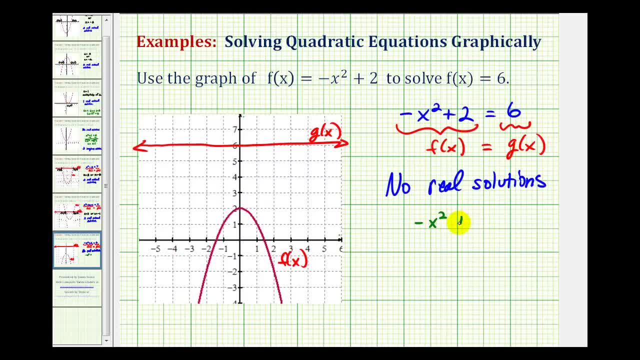 So let's go ahead and do that. So we're going to try to solve: x squared plus two equals six. Let's go ahead and subtract two on both sides, So we'd have negative x squared equals positive four If we divide both sides by negative one. 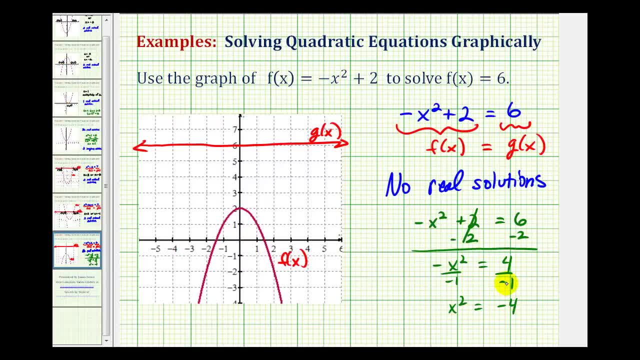 we would have: x squared equals negative four. And now, if we take the square root of both sides of the equation, we'd have a plus or minus sign here. We would have: x equals plus or minus the square root of negative four. Well, the square root of negative four is equal to. 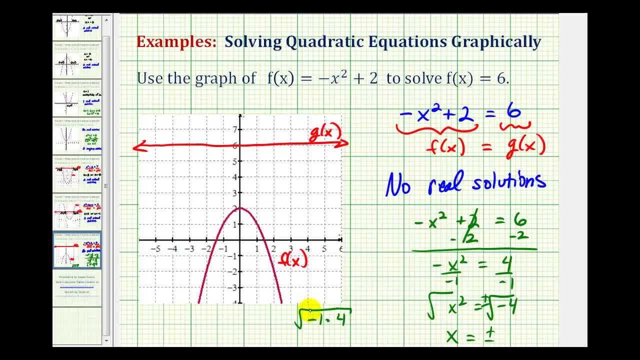 the square root of negative one times four. Well, the square root of negative one would be i, The square root of four would be two. So we have x equals plus or minus two i, which are imaginary numbers, And that's the reason why we did not have